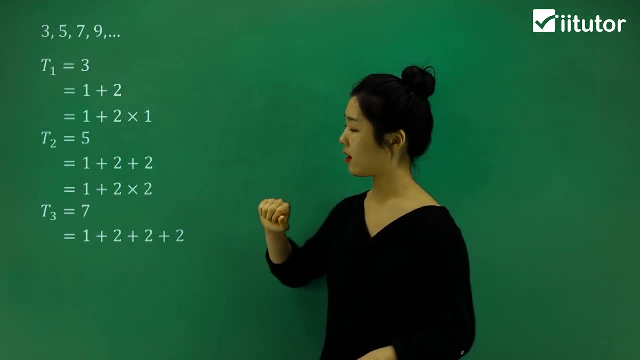 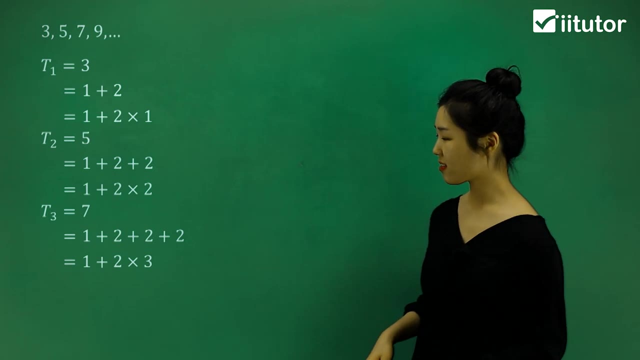 term. I add just one lot of two to one. So you you have three lots of twos here, which means it's two times three. So can you kind of see the pattern now, guys, You can see that to one we're adding how many lots of twos we want. So again, let's try. 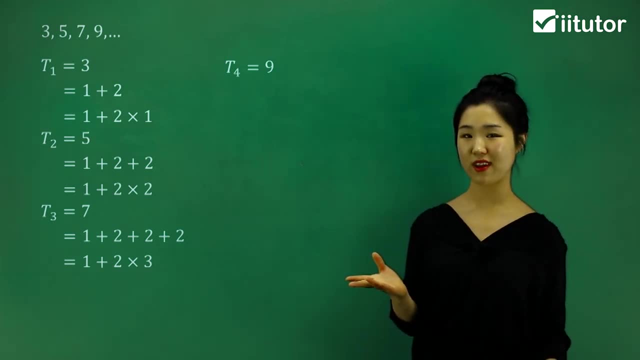 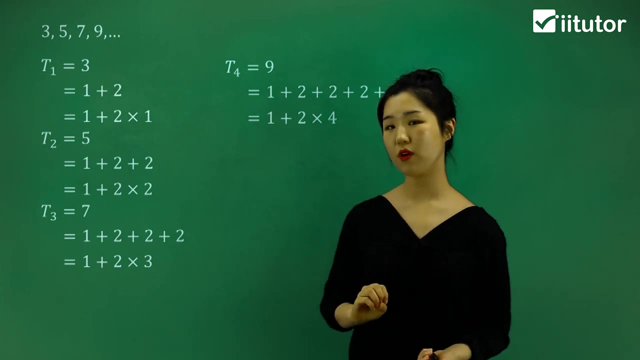 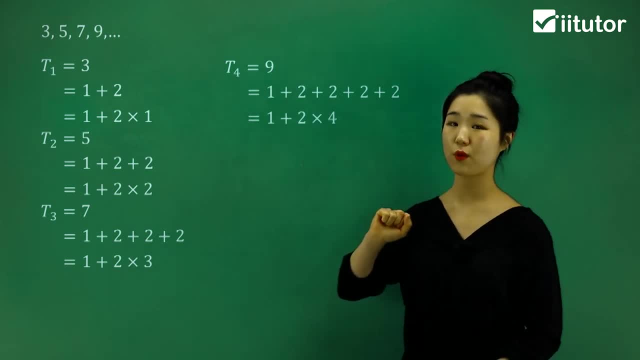 two lots of twos we're adding, three lots of twos we're adding and four lots of twos we're adding. So I'm assuming you guys know how to do next Term five, we'll have to add five lots of twos to one. So that's the pattern. guys, I wrote a general. I'm going to write a little. 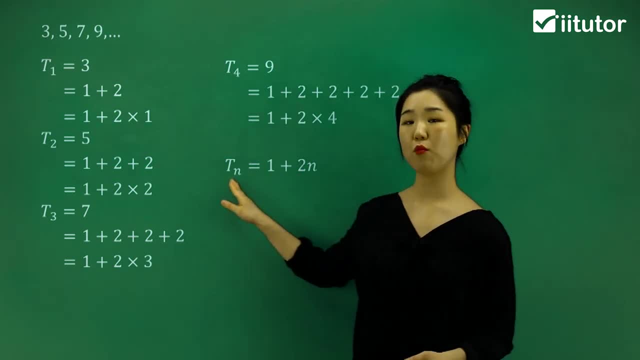 general rule for this. So whatever term, whatever nth term we want to look at, so I'm going to write it as tn. So I mean n could be 10,, n could be 50,, n could be anything. Whatever term we want. 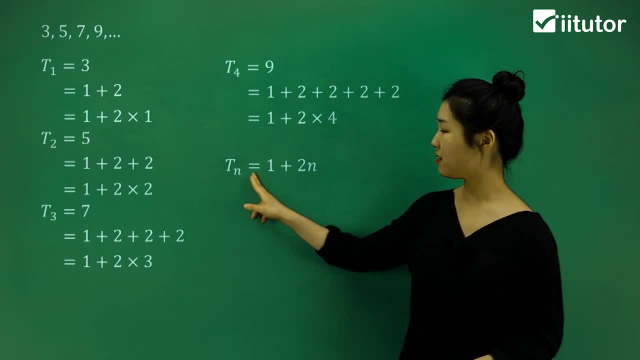 we don't know, we'll just write n. So whatever term, tn is one plus. So see how the pattern was just adding from one, So one plus two times two. So that's the pattern. So I'm going to write a. 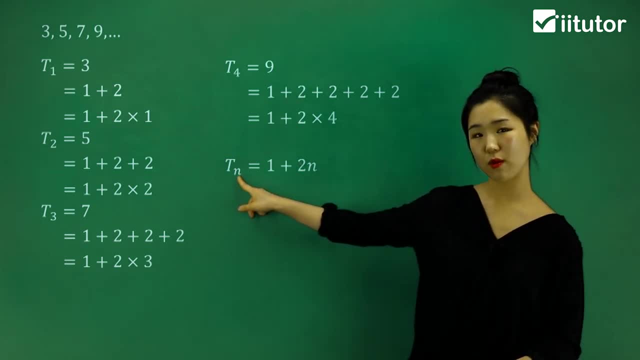 three times as many numbers as what n is. Okay, guys. So see, for this third term we added three times. That's what the rule is. That's called the general term, So, and you can write like this as well, like in a little parentheses, like that, in these little squirrelly brackets, that also kind. 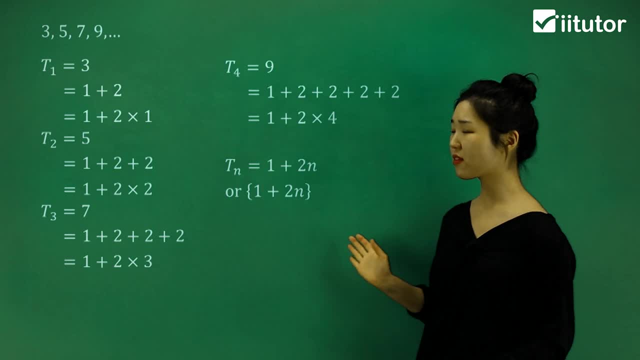 of expresses the general term. So this is how we do it, But the next few questions I'm going to actually give you what the general term is and it's your turn to try and find what those particular values are. So I'm going to write a general term and it's your turn to try and find what those 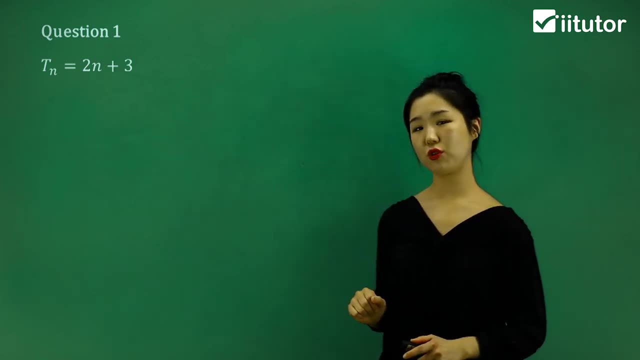 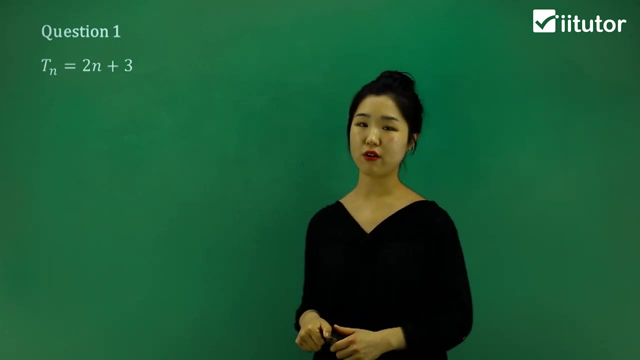 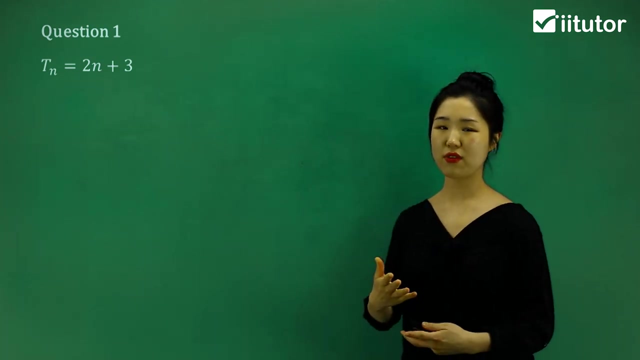 particular values are. So I'll show you. We'll go straight to question one: tn equals to two n plus three. So this is a general term, This is a rule, or specifically the general term of a particular sequence. And see how it says tn. So it gives us the nth term. So if you want the 50th term, 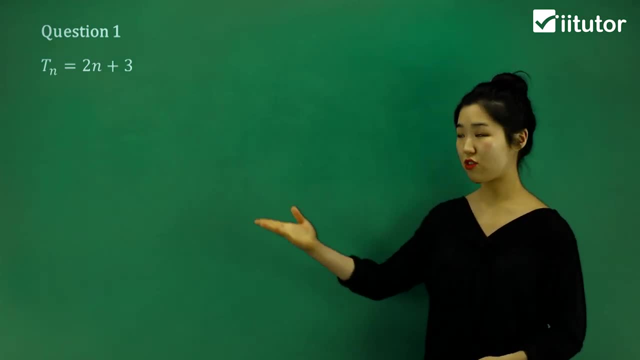 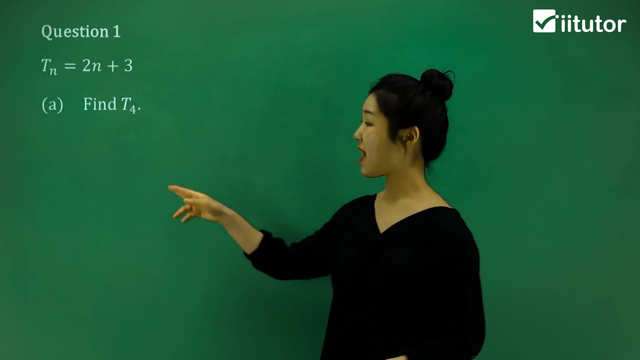 you're 750.. If you want the 100th term, you're 700.. You'd get it straight through that general term. So question one: it says find t4, which means find the fourth term, which means and see.